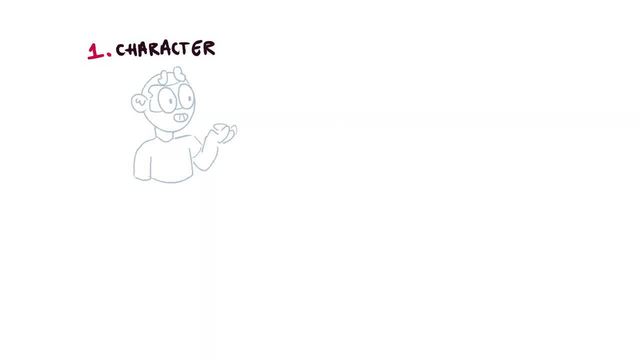 techniques. With that said, here's what you'll need to get started: A character design that represents the narrator, an idea of how you'll transition to and from the story, This one's optional Audio of your story, and a story idea and a super rough storyboard idea. So let's do. 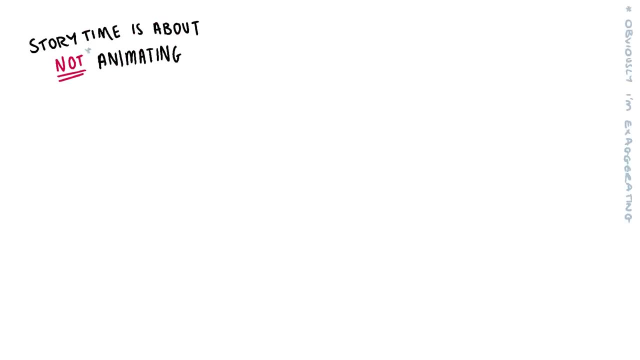 the character. first Story time animations basically aren't animations. You just pop your character between a few poses And throw in the occasional bits of actual animation to trick people into thinking you've done loads of animation. So I'm going to make a new graphic symbol and create a bunch of blank. 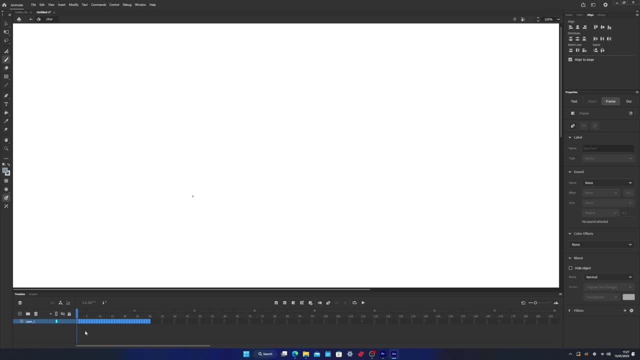 keyframes. On each of these keyframes, we're going to add a pose for our character. Some basic ones might include talking, making a point, really making a point, satisfaction, laughing. I can't believe I did that. I really can't believe I did that. Let's look at the story. 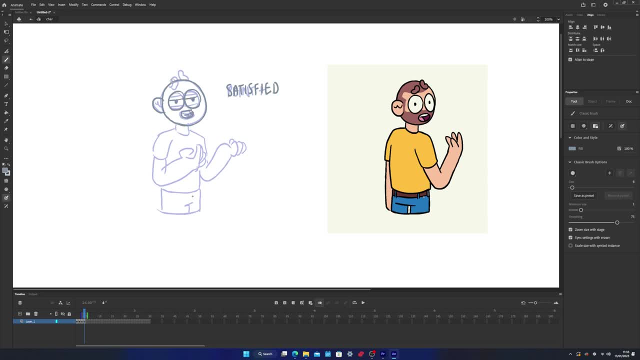 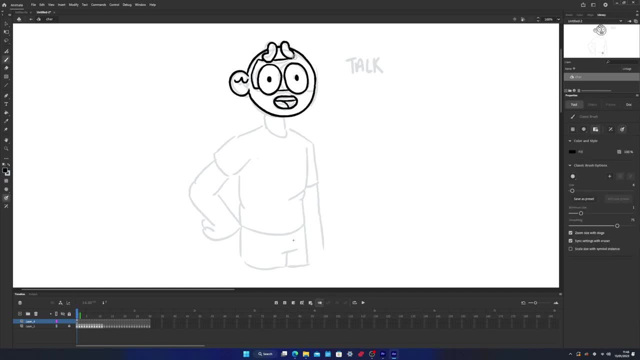 You can do as many or as few as you want, But bear in mind, the more you do up front, the less you have to add later. If you need to come back and add more later on for specific scenarios, just add more frames to the end of your graphic, so you don't mess up any of your 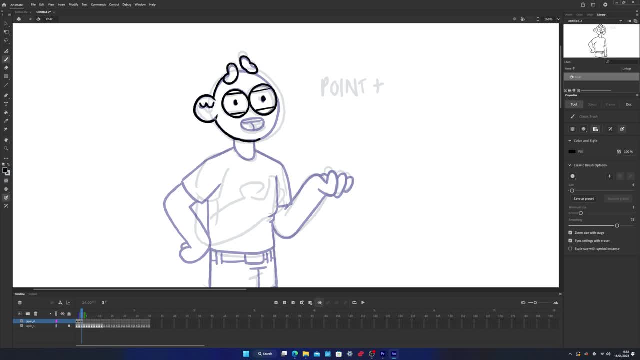 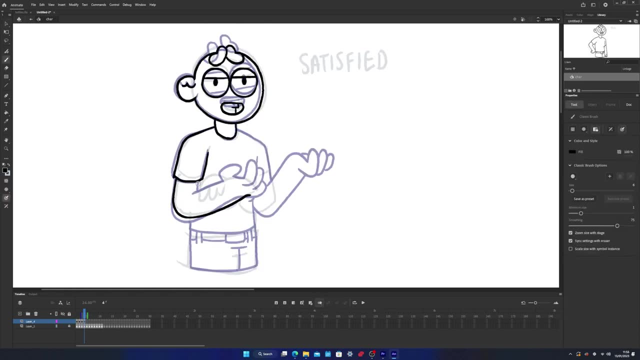 existing animation. Keep the character design simple and tidy up your sketches until you're happy with the design. Once you've made that, stick it aside. for now It's safe in the library. Now you've got your character graphic you can use for every future storytime animation. 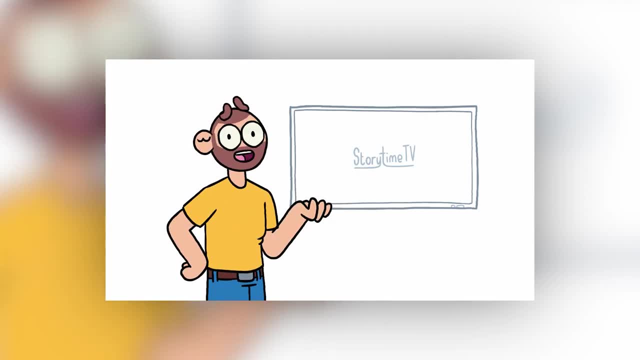 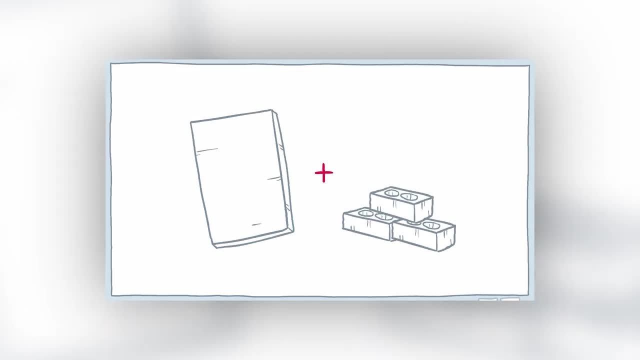 I like to frame my stories so I can dip in and out. This way I don't have to animate the narrator the whole time. In this example I use a story vision TV. When introducing the story, I have the character narrate, then turn to the TV. When telling the story, I cut to the TV full screen. 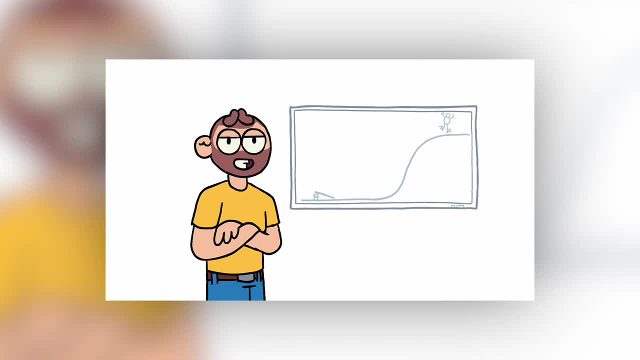 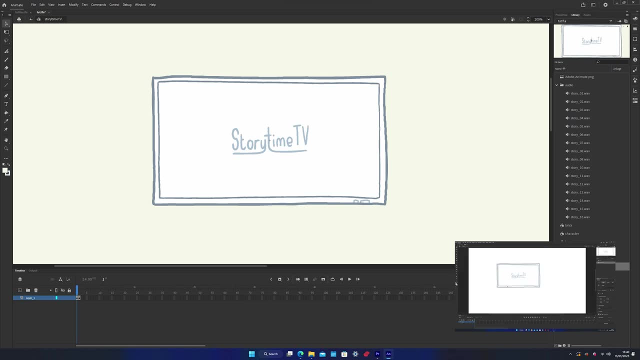 Then you can cut back out to over the shoulder shots of the narrator for comedic effect. So for this you just need two assets: A graphic of the TV on the wall for the narrator shots and another graphic for the full screen story. This can just be a simple. 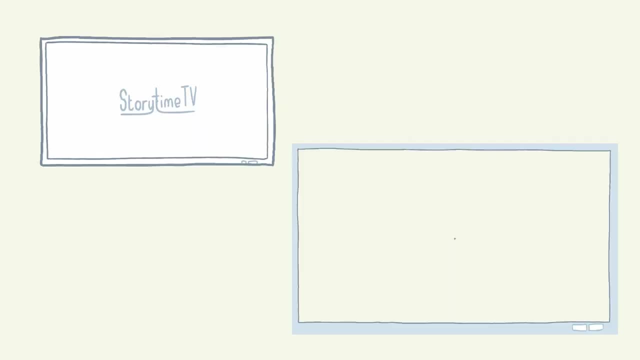 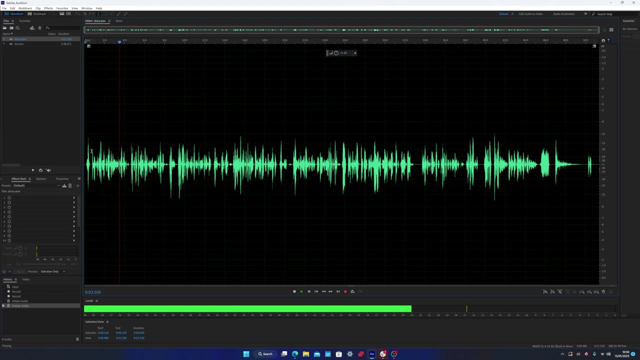 border slightly smaller than your stage. Once they're both made, just leave them in your library. for now, Let's move on to audio. For the audio of the story, I just record it in Adobe Audition, but you can use any audio recording software. Audacity is a good free choice. One thing I'll 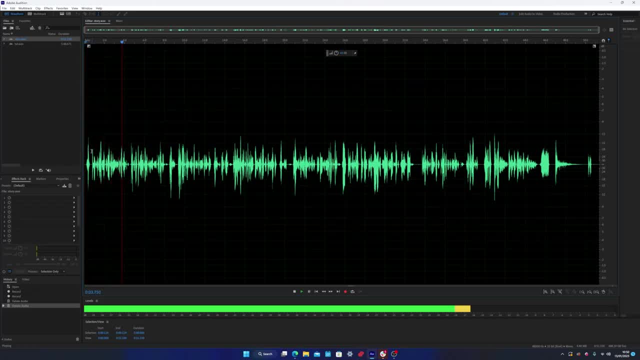 say for Animate is that it's not great for audio editing, so you'll want to break up your audio into chunks to give you more freedom to move them around. once you get into Animate In Audacity, I just record the audio, make sure it sounds ok by applying the podcast voice effect, then select. 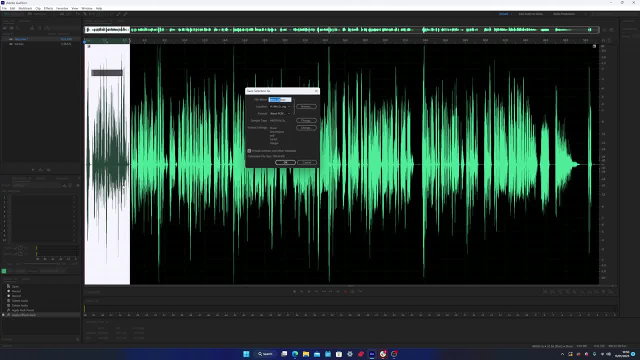 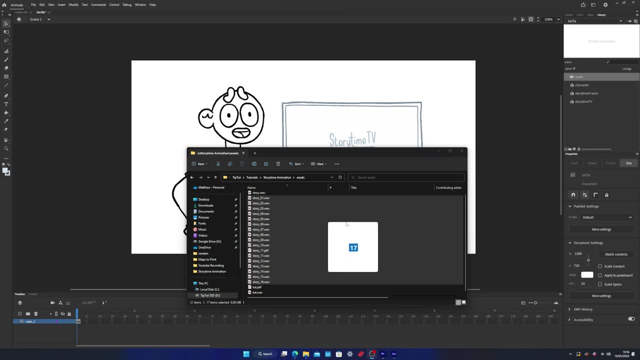 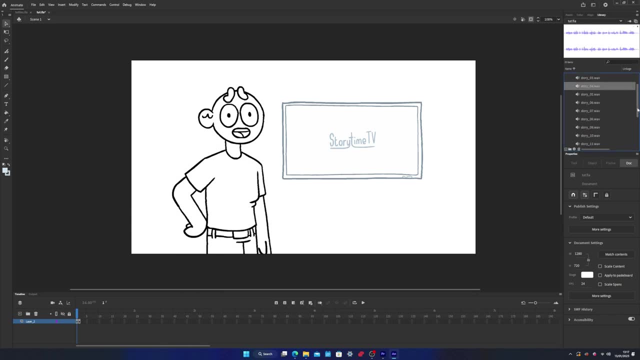 a section, right click, save selection as file. I do this for every natural break in the audio so I can tweak when I get to Adobe Animate, Save as either wav or mp3, then drag the whole bunch into your library. If Animate doesn't like one of them, use the other one, but they should both work. 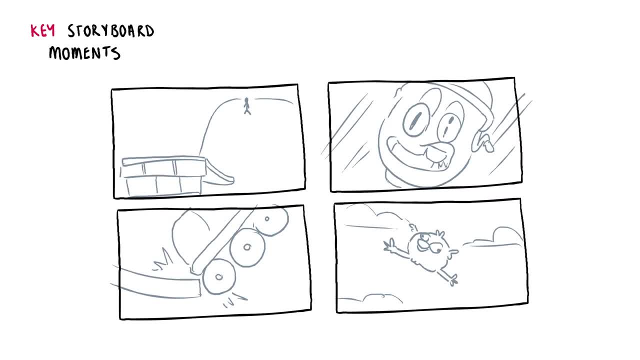 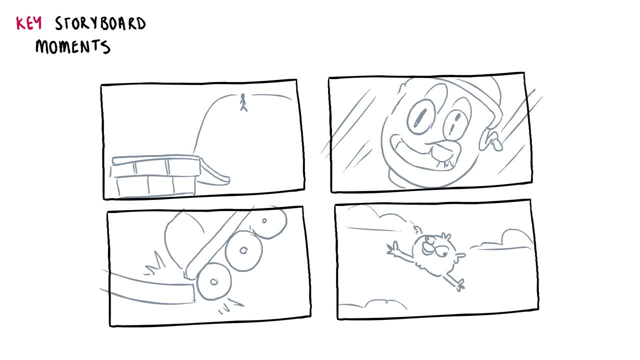 Last step before animation: the storyboard idea. Honestly, I just have an idea for a few key frames in my head, then I just go for it. That's the beauty of storytime animations: you don't need a lot of planning, as the hard part of animating the narrator is already done. 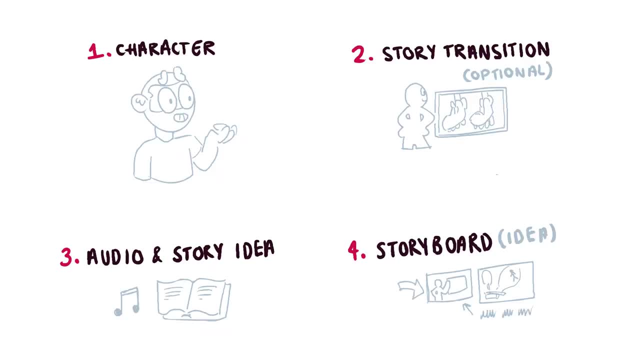 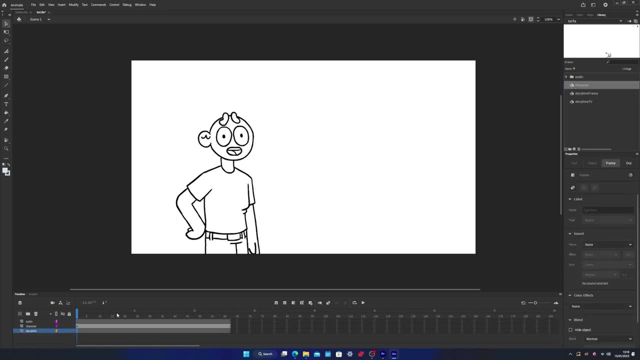 before you start, Just do a quick sketch of the important bits. Now that we've got all the parts, it's time to put it together In a blank document. put your character on one layer, your framing device on another and your audio on a third layer. 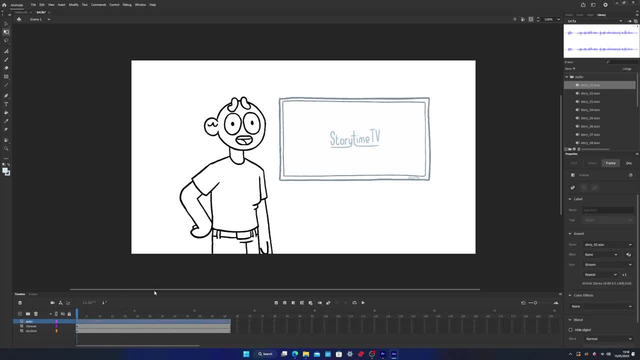 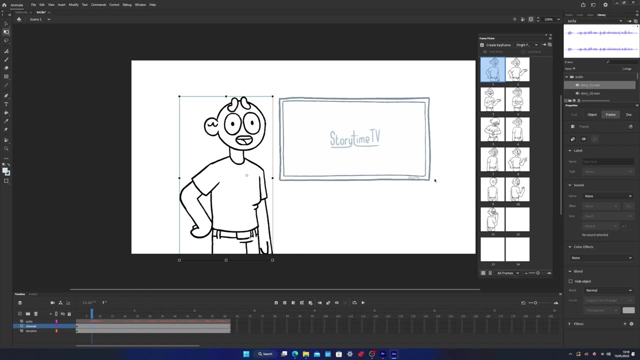 Drag in your first chunk of audio and set the audio type to stream. Take your character and change the graphic looping properties to single frame. Then choose your starting pose. Now go through your audio and change the pose to the one that feels right as he talks, adding a new keyframe each time and clicking the pose in the looping panel. 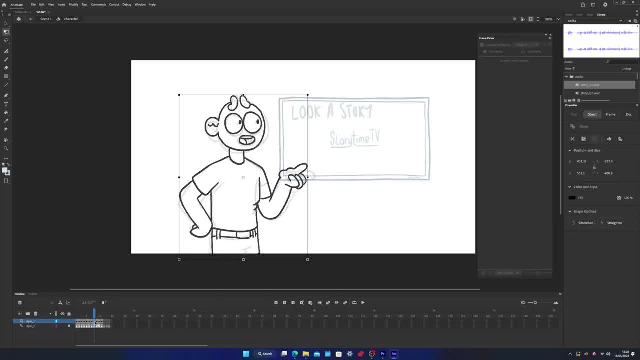 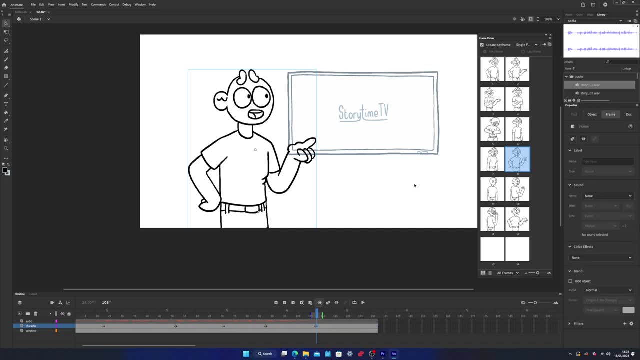 If you find yourself needing a new pose, just double click to enter the graphic, draw the new pose, then exit the graphic and pick the new pose from the looping panel. Now comes the animating. I've covered this in detail before in my bounce technique video. 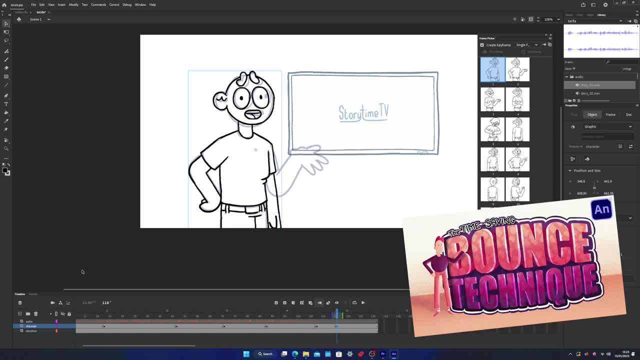 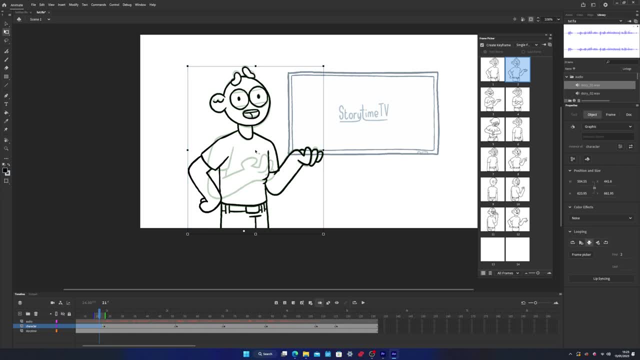 but essentially we'll place a keyframe just before the pose switch and then select the transform tool and, making sure the anchor point is at the bottom of the character, We squish them down a bit and make them wider, Then place the keyframe after the pose switch to basically save the finished. 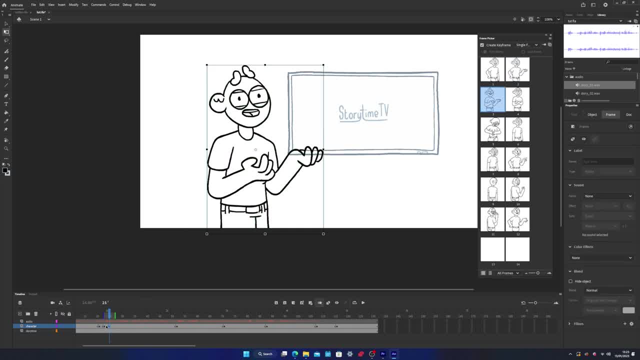 position and then, as you go along, we've got a section onнимating the character and go back to the original pose, switch and stretch them up a bit to make them a bit thinner. You can add some more keyframes to help ease this motion, if you want.